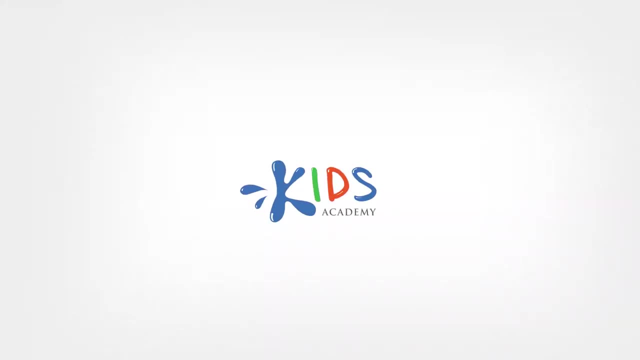 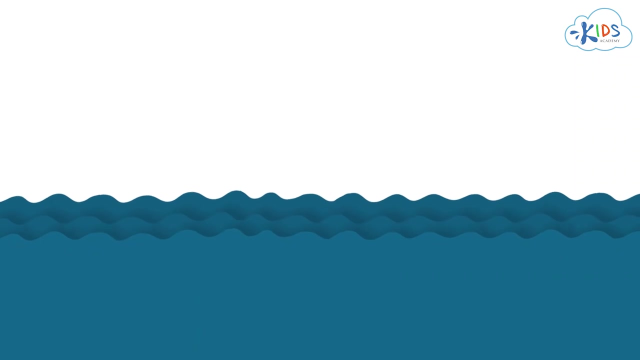 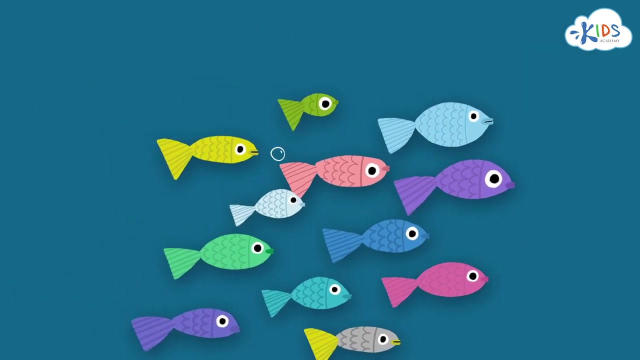 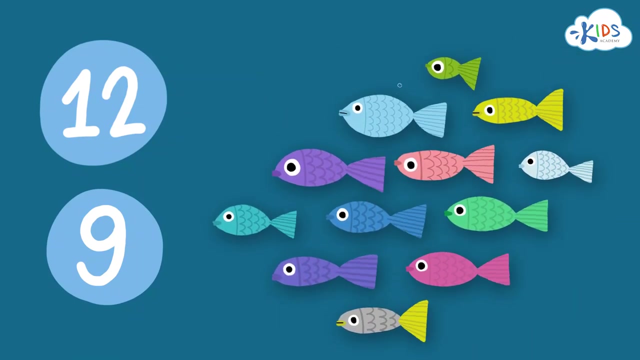 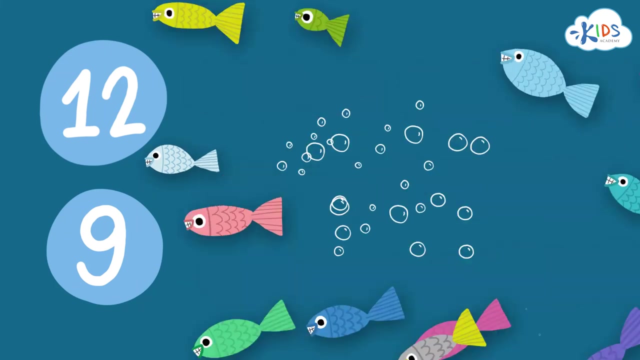 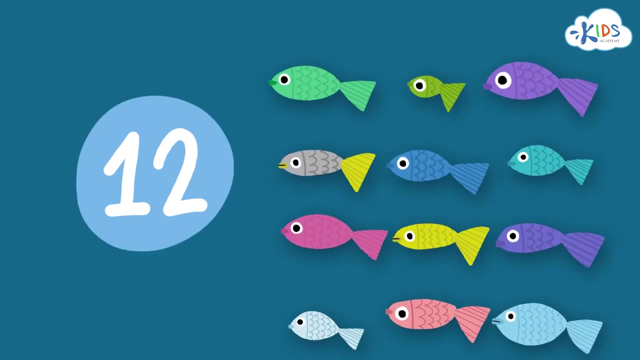 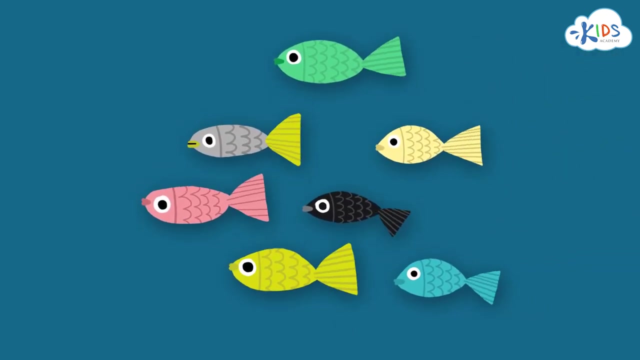 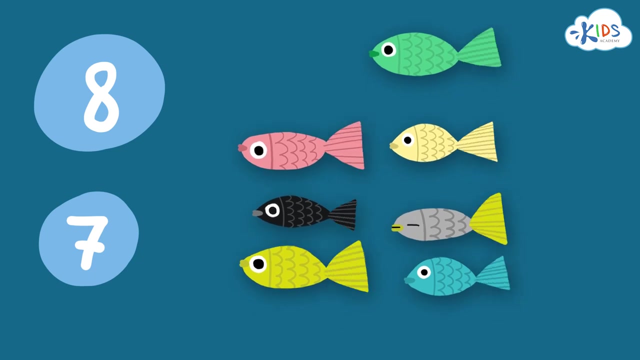 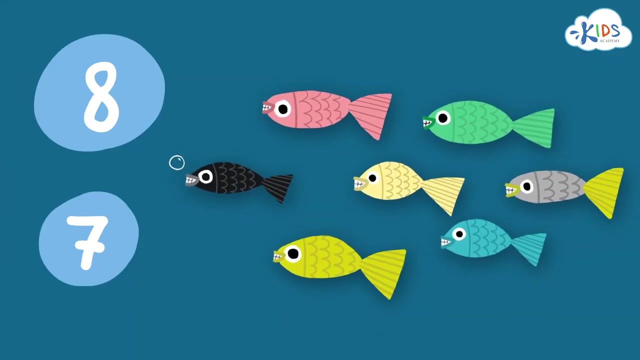 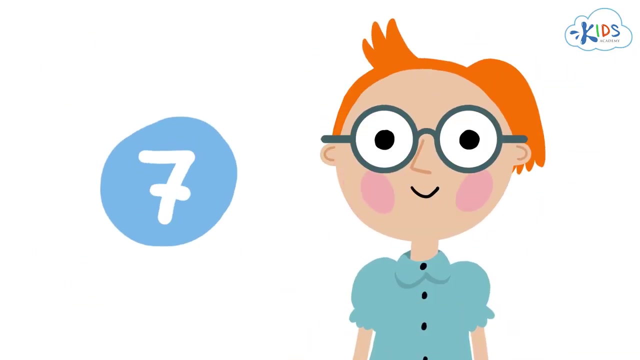 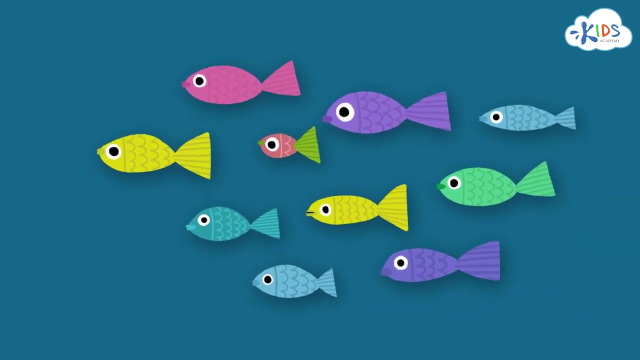 Welcome to Kids Academy. There were twelve fish in the sea. Counting and matching is really fun And it's easy to do. How many do you see? How many do you see? How many do you see? There were seven fish in the sea. Counting and matching is really fun. 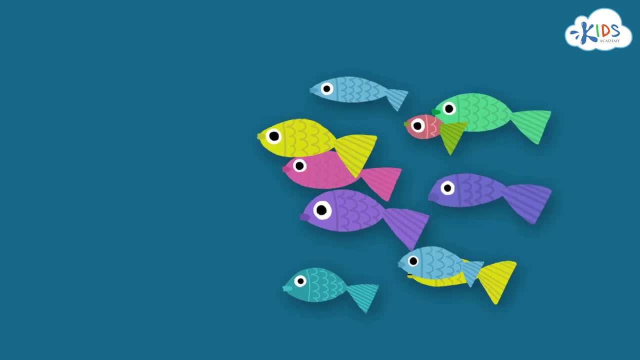 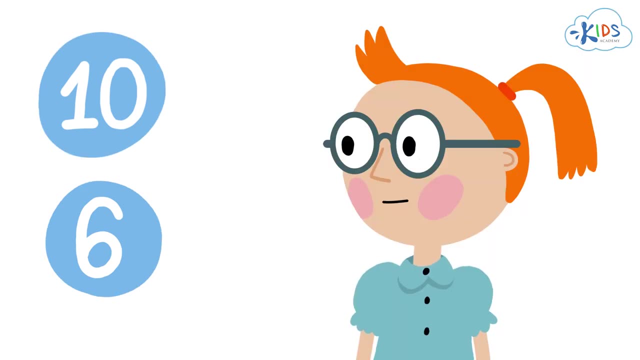 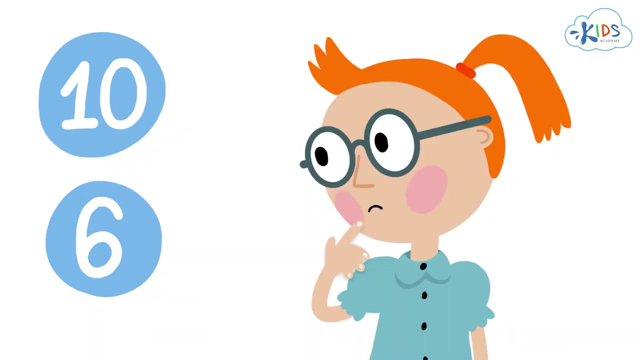 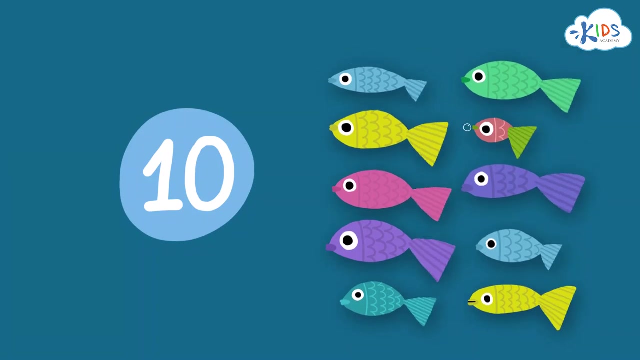 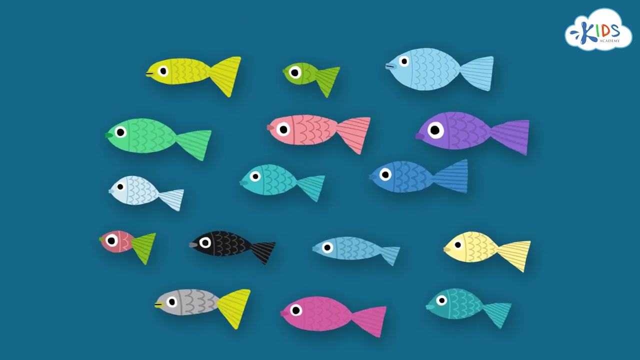 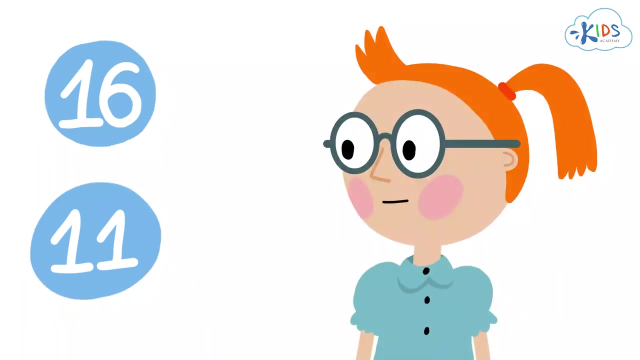 And it's easy to do. How many do you see? How many do you see? How many do you see? There were ten fish in the sea. Counting and matching is really fun And it's easy to do. How many do you see? How many do you see? How many do you see? 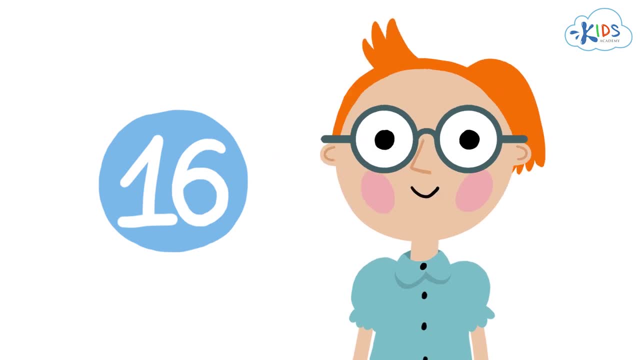 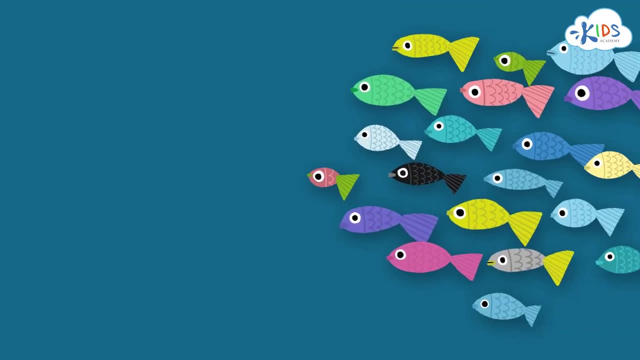 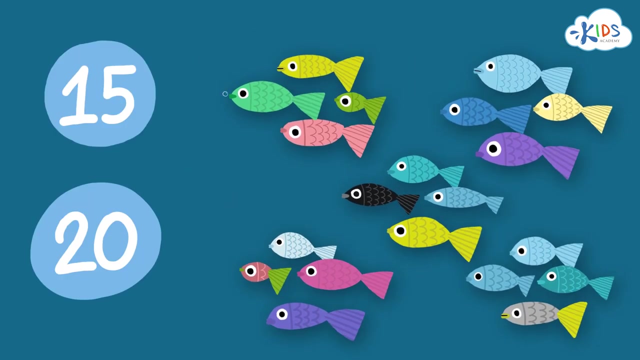 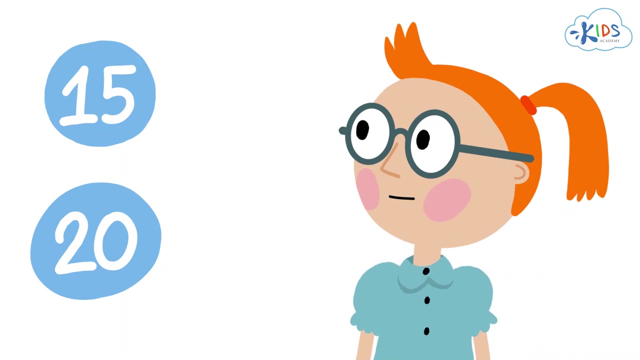 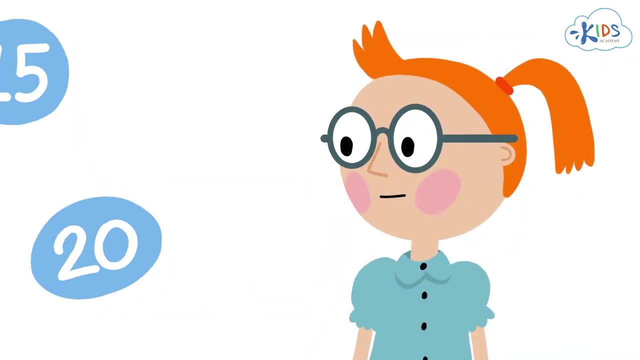